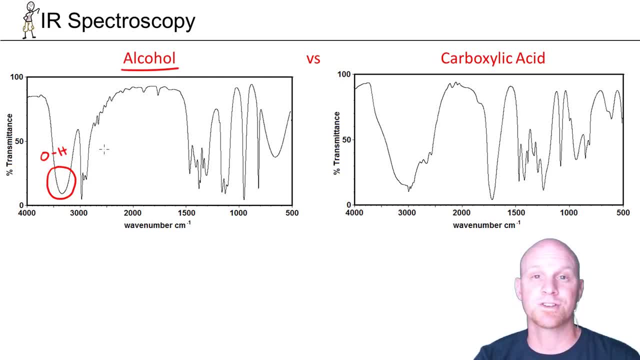 bit ago. it is different in both how it looks as well as where it shifts, than the OH of a carboxylic acid over here. So if you notice, this one centered closer to 3000, but for the alcohol it centered closer to somewhere usually between like 32 and 3600. 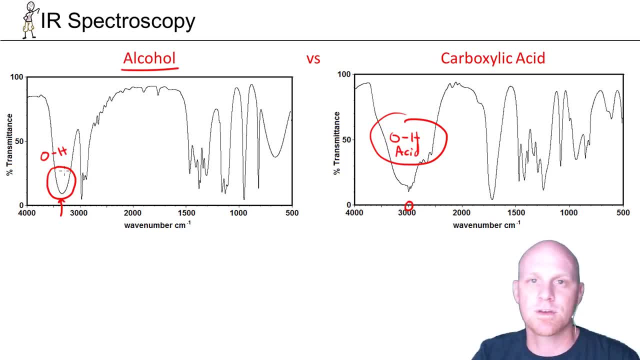 So there's also something you should know. It's so broad, typically due to hydrogen bonding. So hydrogen bonding, it turns out, weakens this bond And so when this molecule is involved in hydrogen bonding with some of the other molecules in the solution, so it weakens. 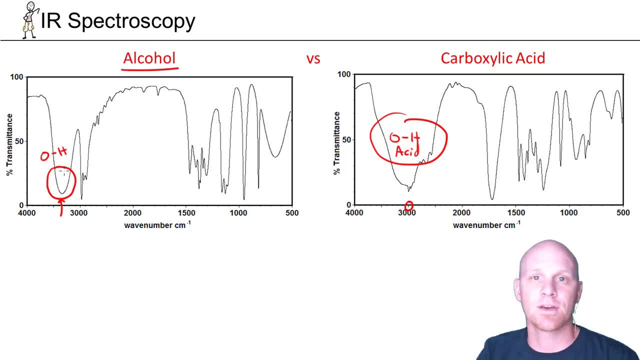 the bond also gives you kind of an average of energies. You get a variety of energies that are possible. So in Azrosa you get a broad peak that's also shifted down a little bit. So if you might make this solution a little bit more, 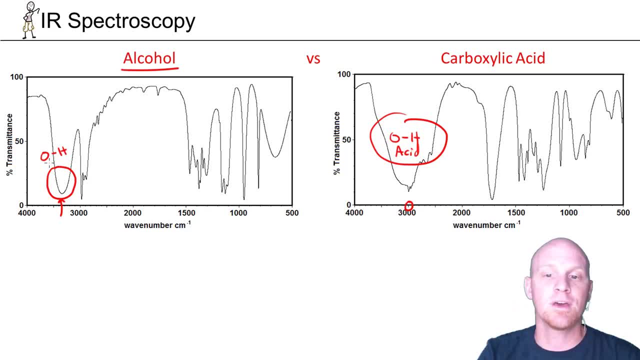 dilute, so there's not as much hydrogen bonding going on. what you'd find out is that this peak might not be so broad and it would probably end up getting shifted to the left Again. hydrogen bonding gives you some average possible energies for the bond vibration. 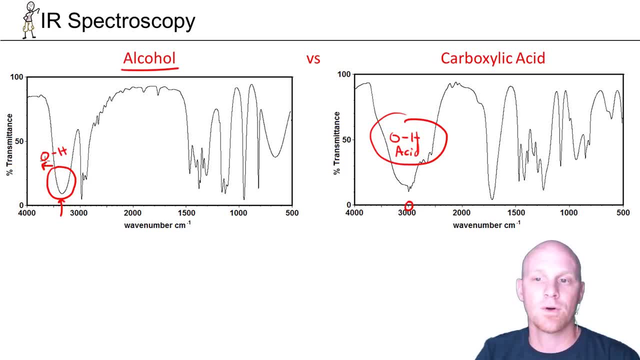 but also weakens the OH bond a little bit as well. So in dilute solutions it'd be a little bit further to the left and probably nowhere near as broad. Just an FYI, But hopefully here you can tell the difference between the alcohol. 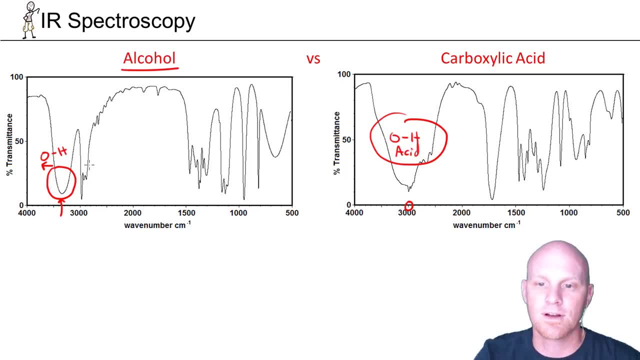 and the carboxylic acid. So if you also look at the spectrum on the left here we've got right here. notice again to the right, right of 3000, these are sp3, carbon hydrogen bonds. So in the spectrum corresponds to some sort of what we call aliphatic alcohol. 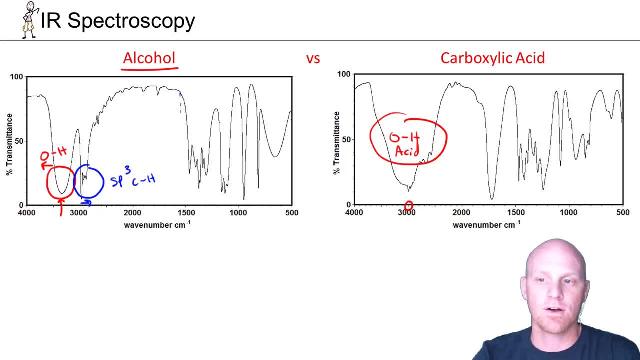 an alkane alcohol and that's about all we determine. Everything else is to the right of 1500, and therefore in the fingerprint region. So again, we're never going to get a complete structure from the IR typically, but I would know this thing's. 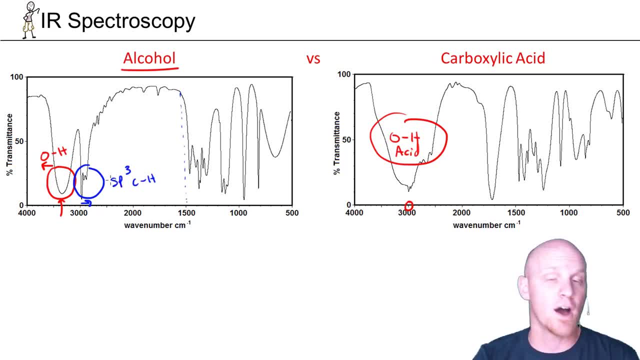 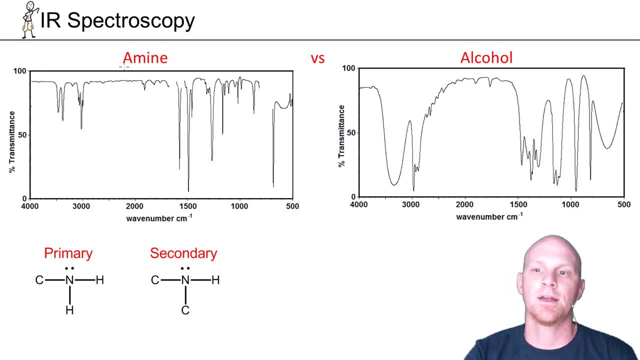 an alcohol and an alkane, and I'd know that it's not a whole bunch of other functional groups as well. So in this next example, I want you to see the difference between an amine and the alcohol we just took a look at. 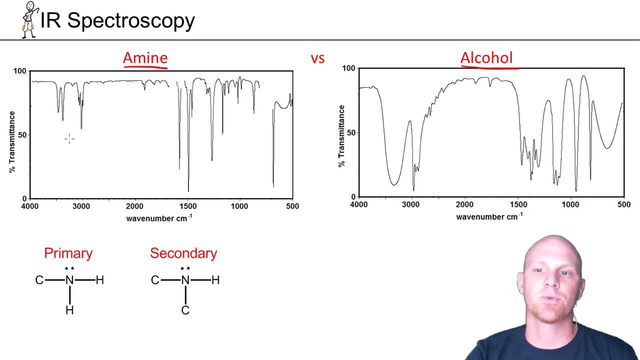 So in this case they both have peaks down in the kind of 32 to 3600 range. So, but you'll see some differences here. So if you recall, the alcohol here is this nice broad peak most of the time. So whereas the amine's usually not quite so broad, it's usually still. 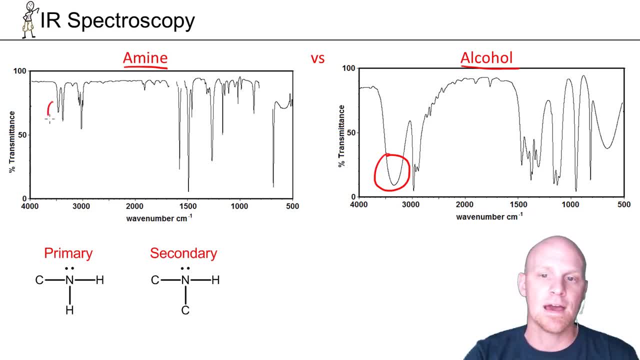 generally classed as broad, but it's not anywhere near as broad most the time And you might see either one peak or two peak, depending on how many hydrons are bonded to your nitrogen. With two peaks we have what's called a primary, either amine or amide. This one's going to be an amine. 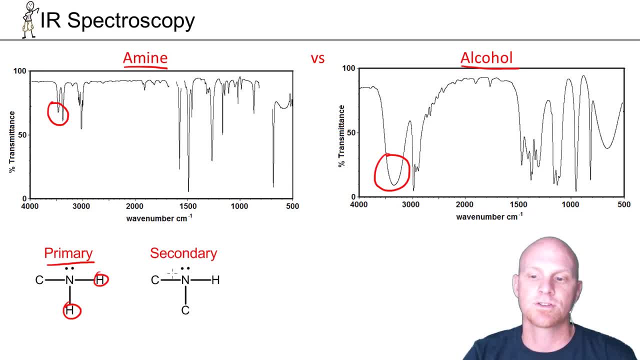 So and that's because the nitrogen's bonded to two hydrogens. So with a secondary amine only bonded to one hydron, you'd only see one of those two peaks actually showing up. So in this case a lot of students get confused at this level- primary, secondary- 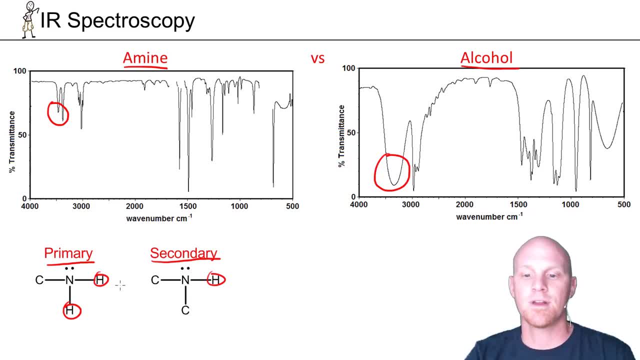 you know I'm confused. So it turns out primary and secondary is determined not based on how many hydrogens the nitrogen's bonded to, but how many carbons it's bonded to. So with this nitrogen being only bonded to one carbon, that's a primary. 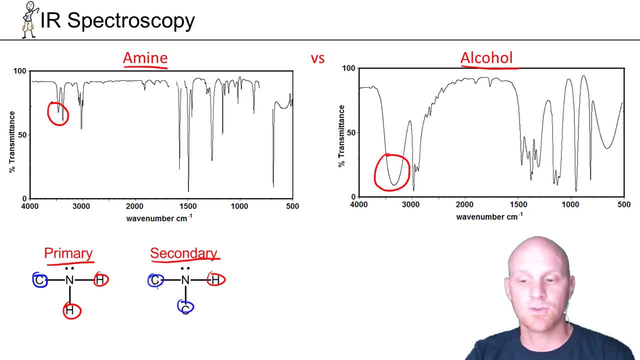 amine, With this one being bonded to two carbons and only one hydron. but two carbons, that's a secondary amine. So if you're confused where that classification comes from, that's where it was coming from. So, but these are the NH peaks, and I'm just gonna say NH2 in this case, since 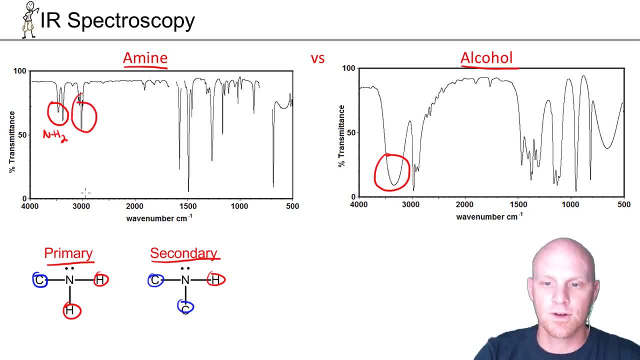 there's two peaks, two H's. So right over here, if you look again right where 3000 is, that's largely to the left of 3000.. So these are your sp2 CH bonds also showing up in this. 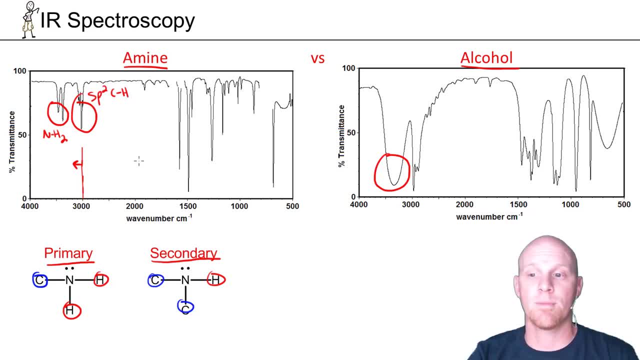 And if we have sp2, carbon hydron bonds, that either means alkene or aromatic. So in going off over here, we've got a couple of peaks right in the 1500 to 1600 range And that's a giveaway. you've got a benzene ring, So it turns out your. 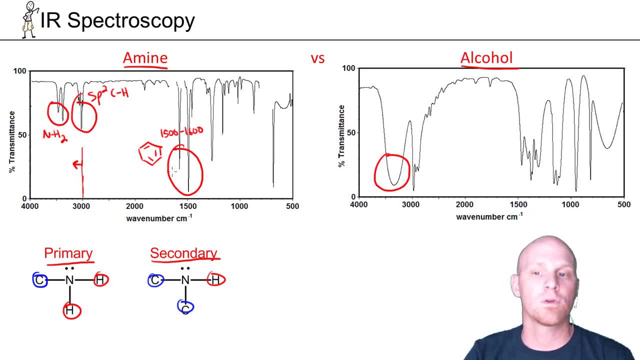 benzene. carbon. carbon bonds generally show up with a combination of one, two or three peaks and kind of that 15 to 1600 range. You'll also see some much smaller peaks, typically in this range, but I don't usually like identifying benzenes from that. 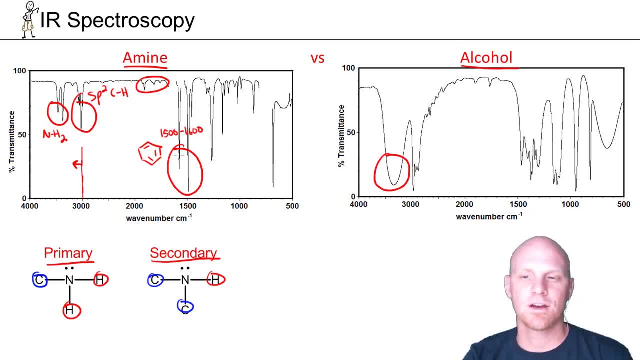 but rather from these peaks from the 15-1600.. When I say 15 to 1600, one thing you should note: it usually means a little lower than 15 to just a little bit higher than 16.. Little bit of a buffer on that, But you might see. 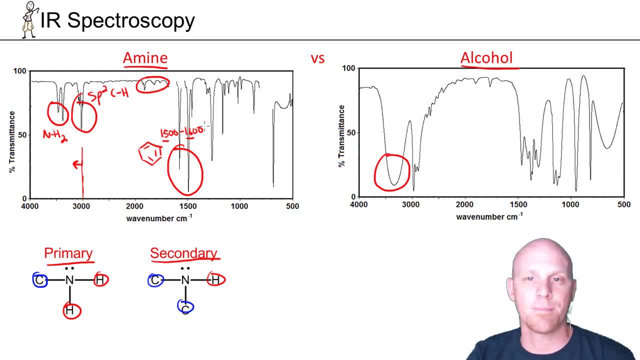 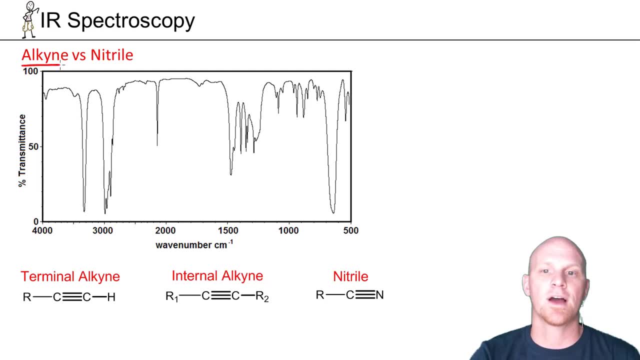 one, two or three peaks, depending on the specific aromatic compound. So the last example we're going to take a look at I'm going to use to help you distinguish between an alkyne and a nitrile, And if you don't know what a nitrile is just yet, a nitrile has a 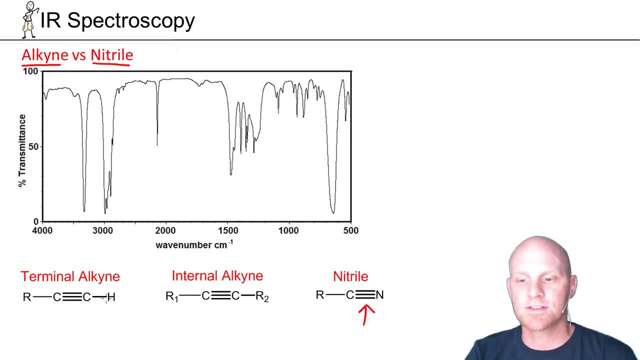 carbon-nitrogen triple bond here. So in this case alkyne has a carbon-carbon triple bond. so, and you might recall, those triple bonds show kind of right up in here in this 21 to 2300 range. So if we look at the differences here there's two types of alkynes. We've got a terminal alkyne. 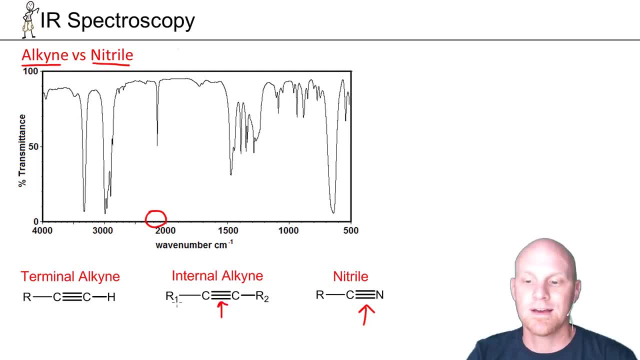 and internal alkyne. and if you recall, with this internal alkyne, if we showed an example of IR inactive bonds involving an internal alkyne, and if R1 and R2 are identical groups, this thing will be perfectly symmetrical. it'll have no dipole moment and, stretching it, it'll still have no. 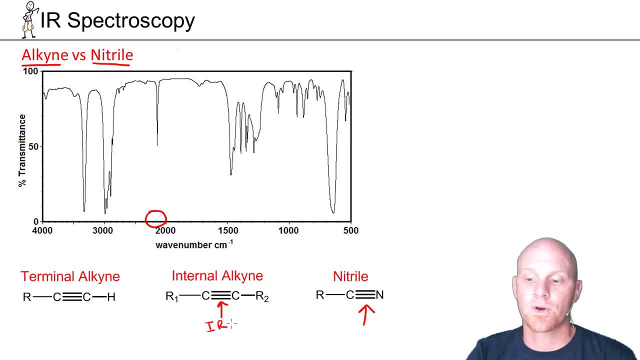 dipole moment and so, as a result, so your carbon-carbon triple bond would be IR inactive. Well, it turns out even if R1 and R2, again still being carbon chains, even if they're not identical, they're still inactive. So, even if they're not inactive, they're still inactive. 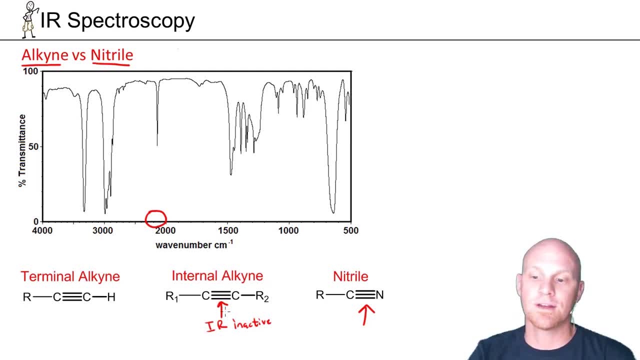 So even if they're not inactive, they're still inactive. So it turns out this thing has such slight polarity associated with it that you don't ever typically get a strong signal for an internal alkyne. You might get a super small signal in that 21 to 2200 range, but oftentimes it's just not. 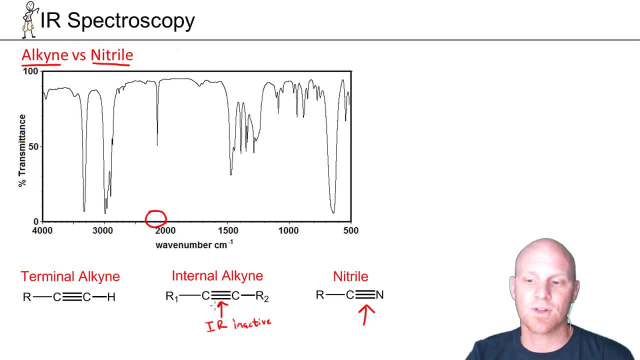 even visible. So even when it's not perfectly symmetrical, you're usually not going to see the internal alkyne, so we'll just kind of ignore it for this comparison. But if you look at the terminal alkyne here, so this molecule actually is polar now with a carbon chain on one side. 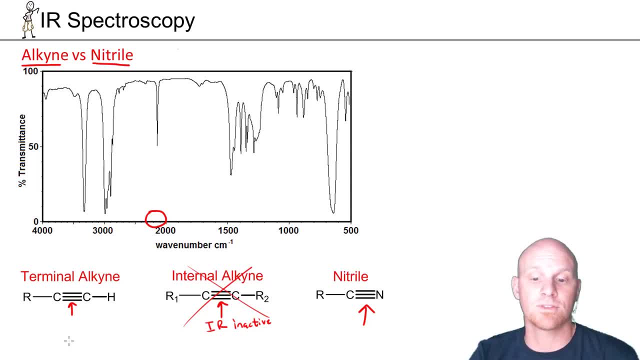 a hydrogen on the other. so and when you stretch it you definitely change the dipole moment. so it's definitely going to show up And again, this generally is going to show up somewhere around 2200.. But for your nitrile it also is going to show up generally somewhere. 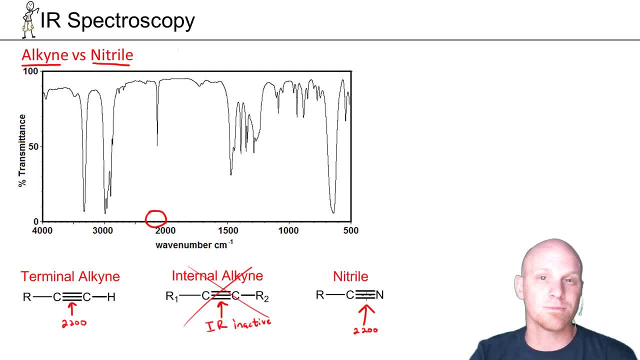 right around 2200.. Now it's a slightly more polar bond, It turns out it might show up just barely further down. slightly higher absorption, higher wave number. It also has a more polar bond, so it might be a little bit stronger absorption, but not a ton there either. 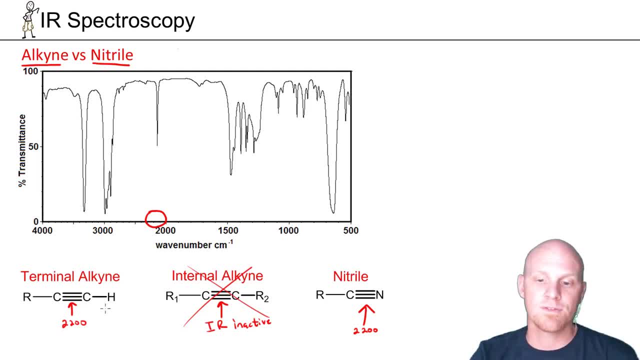 and if you don't have them side by side it might be hard to tell. So the big difference between them then is, with the terminal alkyne you're always going to get additional peak right here for that sp carbon hydrin bond that shows up at 3300.. So if we look, 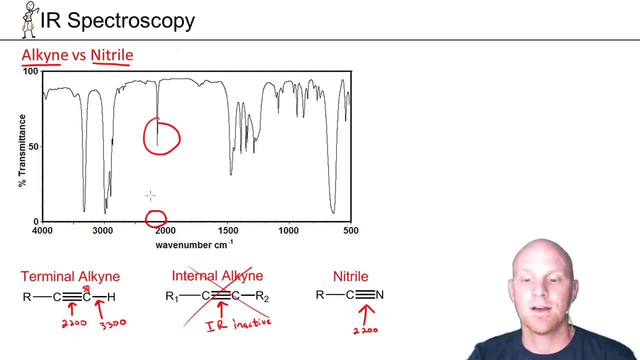 at our spectrum at hand. here again, we've got this triple bond right here and again, whether it's carbon carbon or carbon nitrogen. immediately I look over at 3300, and we have this nice, lovely strong absorption That's the spch. and being the spch, it tells me I've got a terminal alkyne. 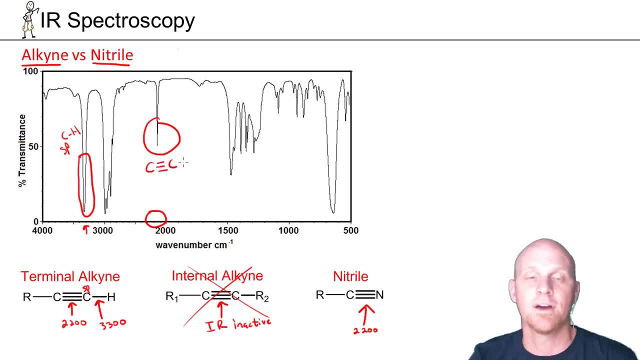 not a nitrile, and so this corresponds to a carbon carbon triple bond, not a carbon nitrogen triple bond. So the other signals again left of 1500 that we might have to identify outside the fingerprint range is just these guys right here and being just to the right of 3000, not just to the left.